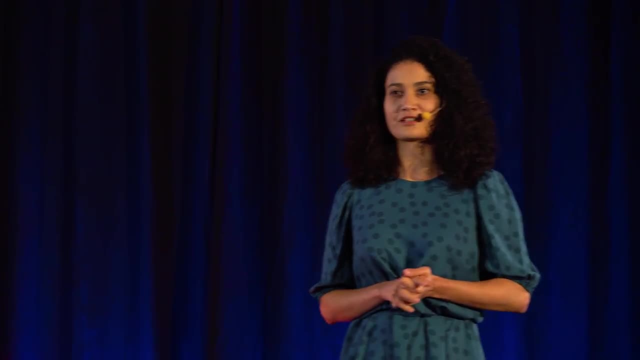 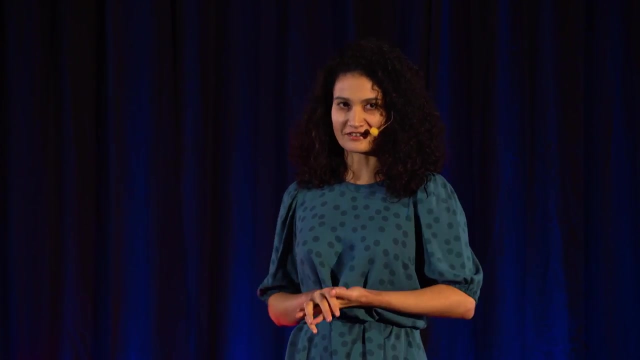 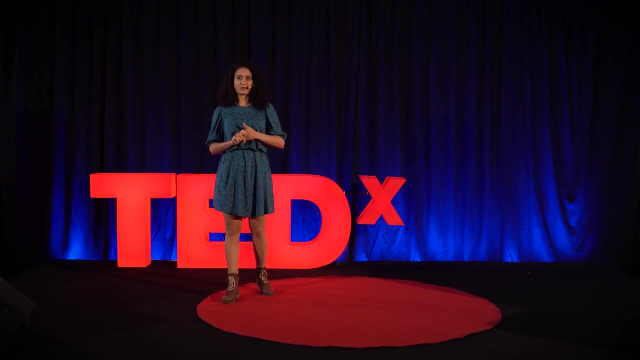 So he opened a bioinformatics group in the Institute of Molecular Biology, the first one in the country to focus on human genomics, and that's where the journey started. However, it was not until I read an interesting paper that I realized the power of bioinformatics. 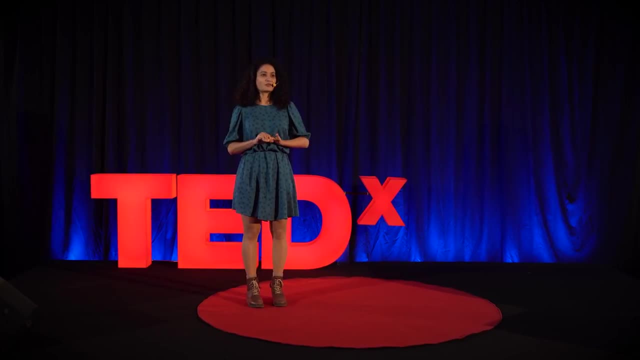 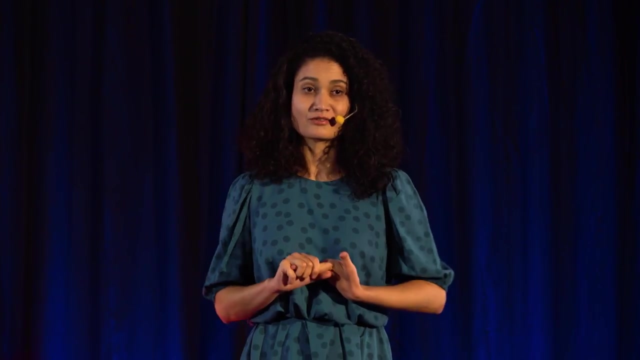 The paper was about telomeres, the biological clocks of our cells. I was interested how they contribute to aging and cancer development and I even had an idea of how to study that. I approached my supervisor, afraid that we might not have the resources to do so. 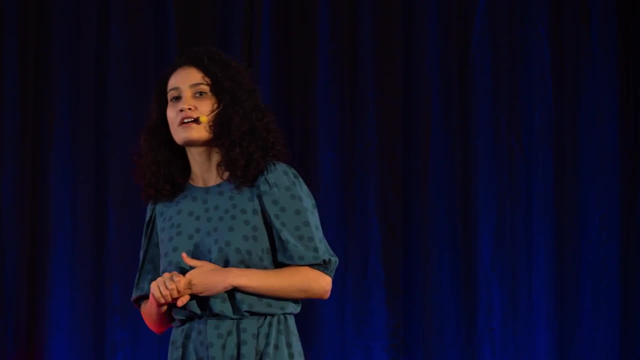 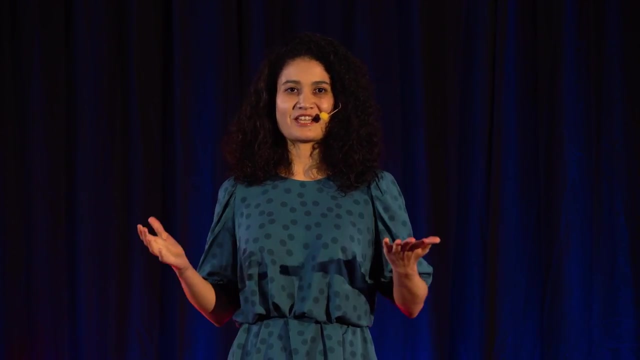 and to my surprise, he thought for a while and said: why don't we download the data from the web and analyze it for this purpose? To me it was a game-changer. It meant that with plenty of data on the web, one can study almost anything. 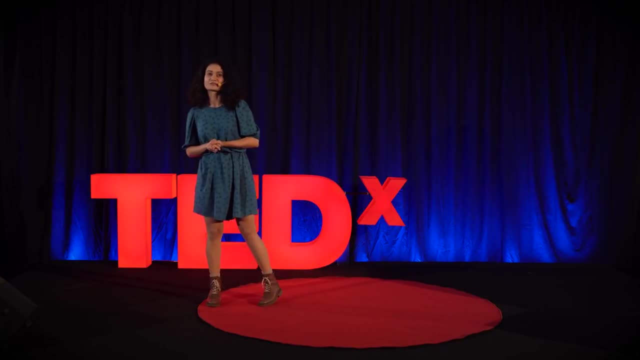 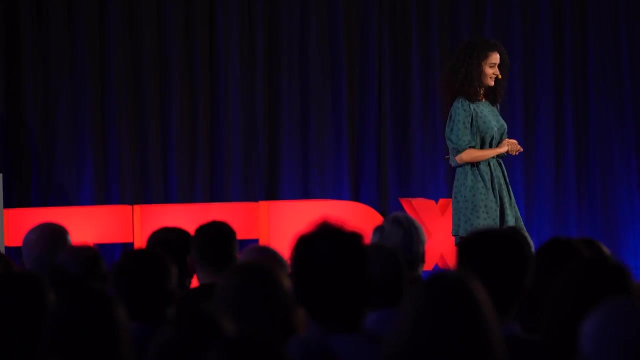 We were among the first ones to leverage genomics data to study the role of telomeres in cancer and in aging and finally we were ready to publish. It appeared that we were not the only ones: A group at Sanger Institute, 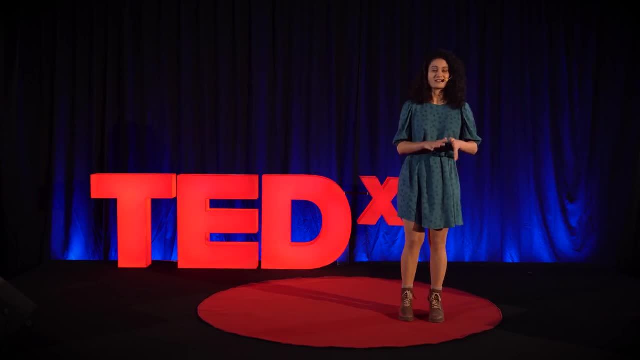 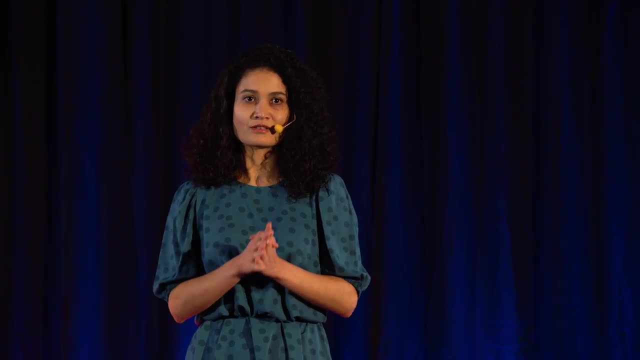 New York-Cambridge just published a paper with the same title that we were going to. Although a disheartening experience in the beginning, it actually gave me a sense of inclusion, Being in the same game with other leading institutions equipped with the same tools as them: computers and imagination. 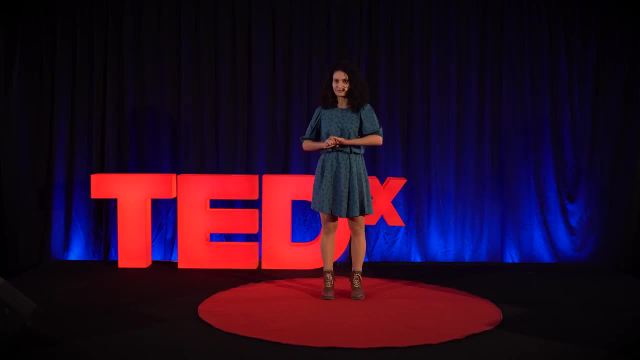 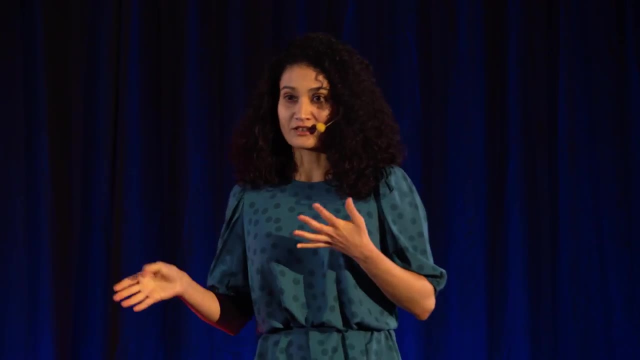 all while sitting in your home country was a dream come true. We eventually published as well and continued our research, including our research on human genomics, Also finding great collaborators, traveling a lot and having fun. I did my PhD on the same topic. 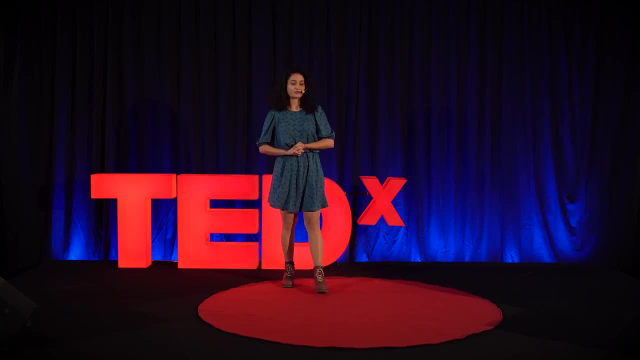 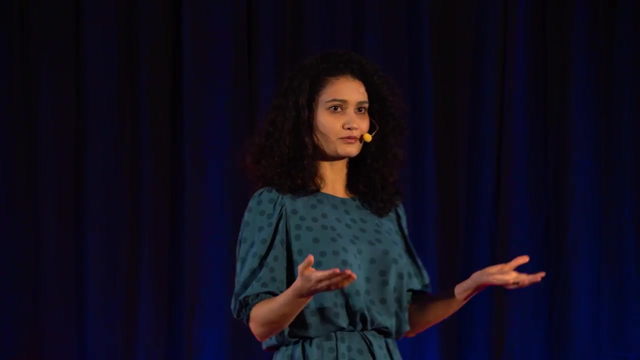 also co-supervised by another great collaborator from the University of Leipzig in Germany, and eventually obtained a Marie Curie Fellowship to conduct postdoctoral studies in Sweden. And now, walking in the streets of Stockholm, I was thinking: if all of this was possible for me, why would that not be the case for others? 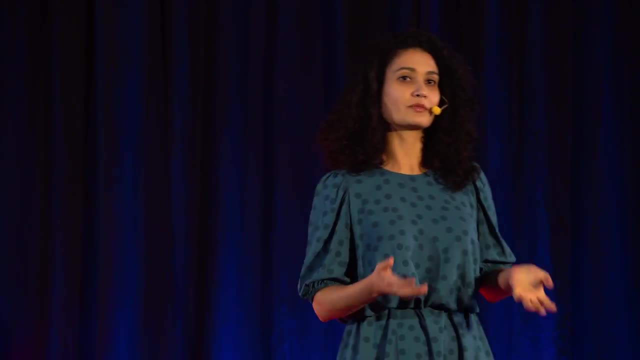 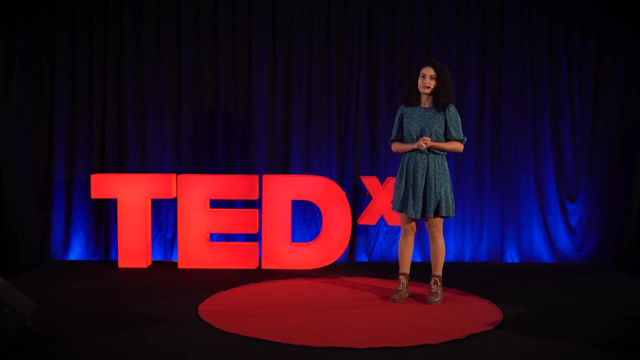 Why would that not be the case for others? My supervisors had opened up the opportunities for me, and that had changed my career path Over the years. a few more students in Armenia had also benefited from that, But the pace of growth was simply not enough. 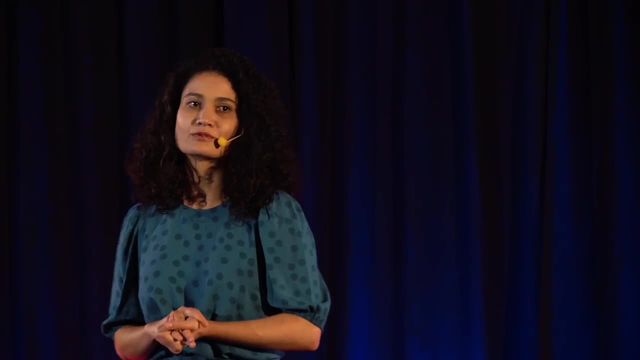 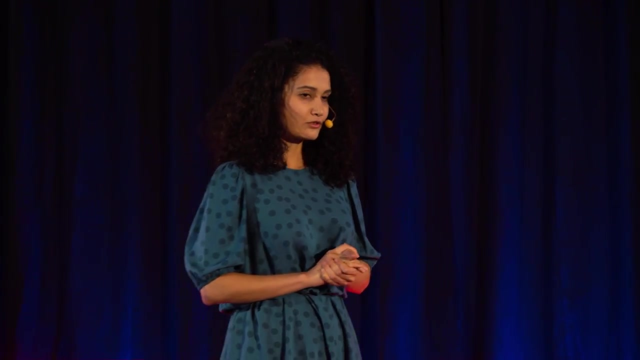 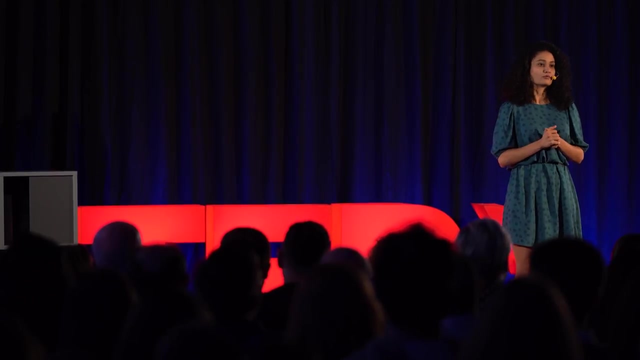 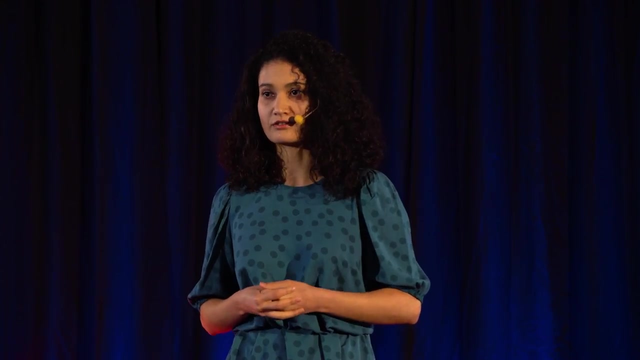 I wanted to expand our activities and engage many more students and show them the enormous opportunities that a career in bioinformatics brings, And this was not just about creating opportunities in vacuums. This was a long-term vision to meet the future market needs that are already knocking on our doors and will be knocking even harder tomorrow. 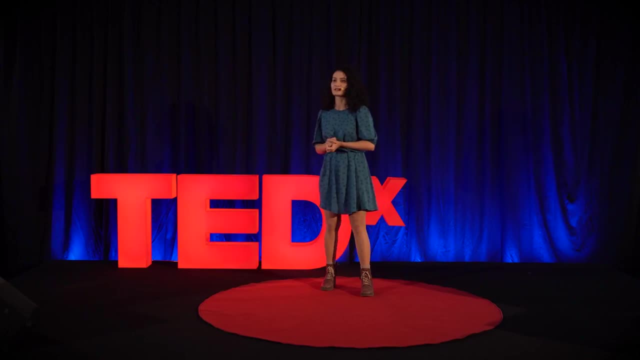 So this is what I was determined to do. when I packed my bags five months ago and returned back to Armenia, I was not alone. My colleagues in Armenia and abroad and many community experts had joined the call, And shortly after, the Armenian Bioinformatics Institute was officially established. 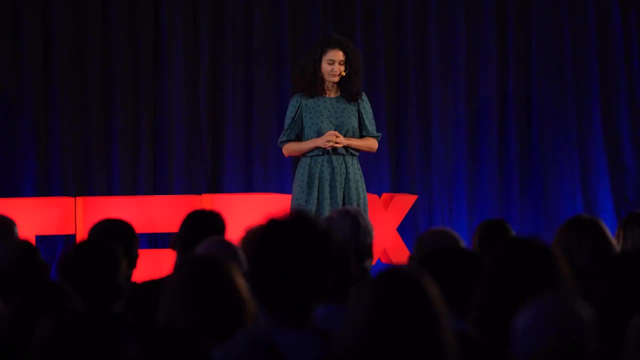 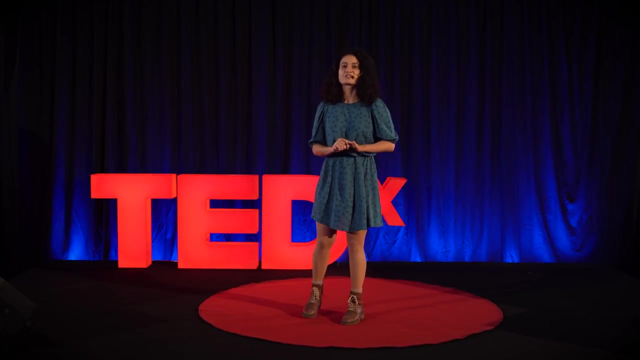 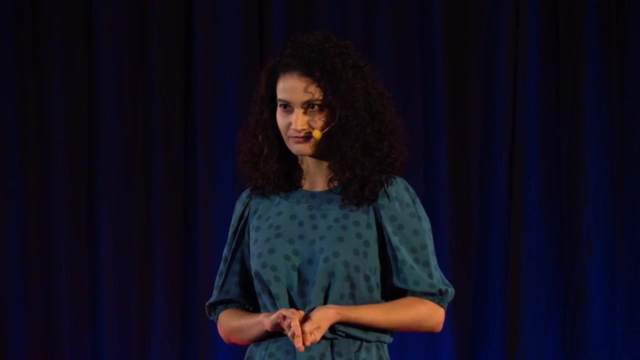 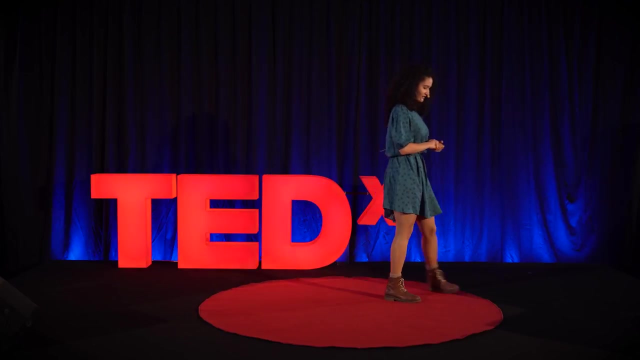 as a non-profit scientific educational foundation. Our mission was simple: Create the human capital that would eventually drive developments in the genomics-heavy biotech sector. But where do we start? Should we start from the universities? Well, we've learned the hard way that in a country with no relevant marketplace. 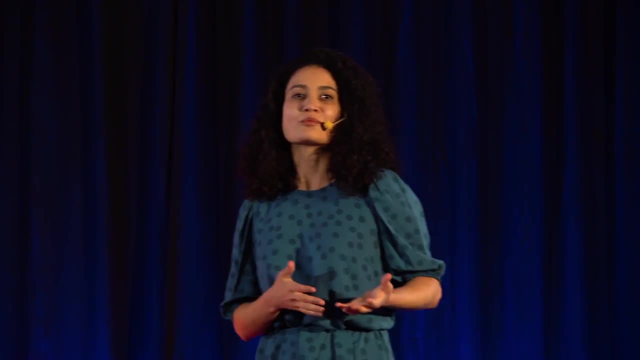 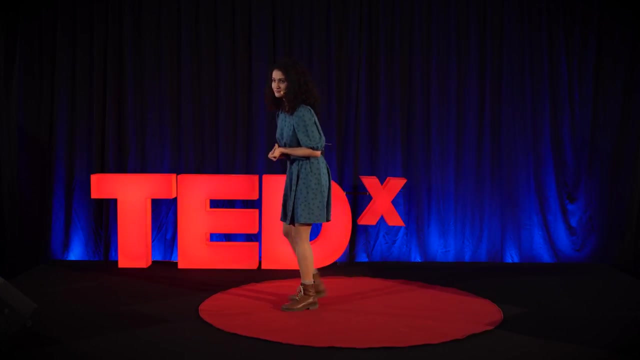 to drive student admissions. establishment of a separate educational program is simply not feasible. Should we start from the industry first? The answer, as you guess, is again, it's not feasible. Why? Because, as you heard in the introduction, the number of genome bioinformatics experts with a PhD degree in Armenia 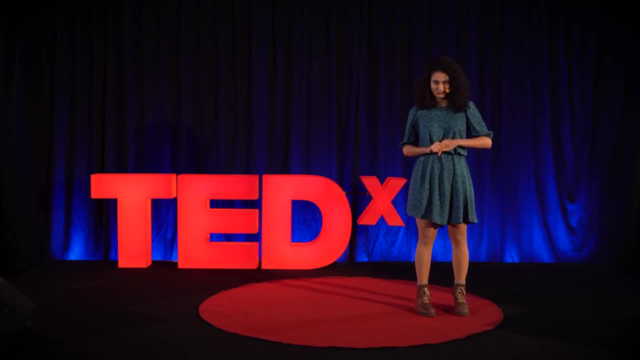 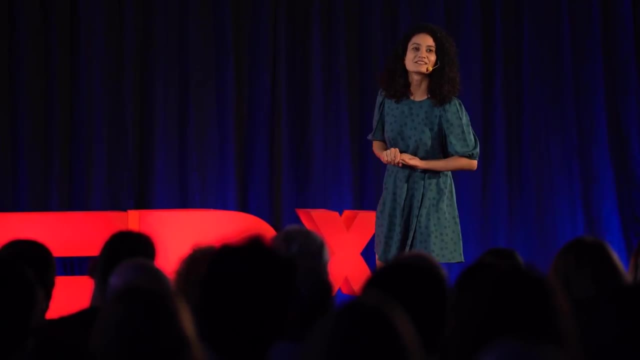 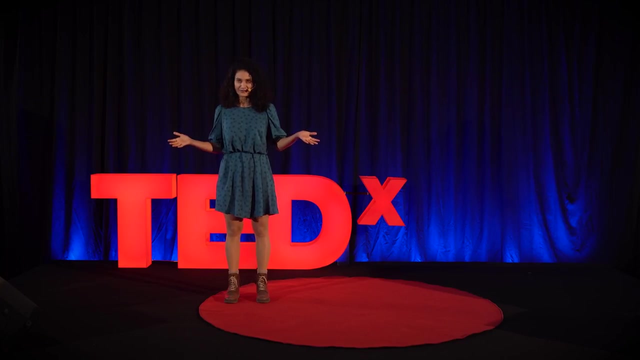 is pretty funny. It's just two, Including myself. if you were wondering What is possible to achieve with this, number Two was the number of individuals from each species that Noah had put in his ark. Sustaining a species with just two individuals is maybe possible. 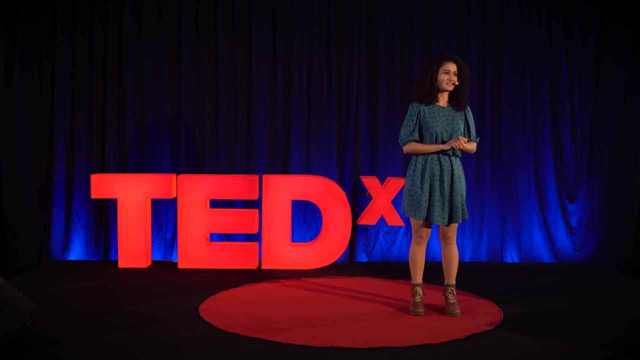 heavily dependent on chance, but nevertheless possible. But believe me when I tell this, bioinformatics is a bit harder than just reproduction. And even if it's possible to do research, sustaining an industrial ecosystem with just two people is simply not serious. 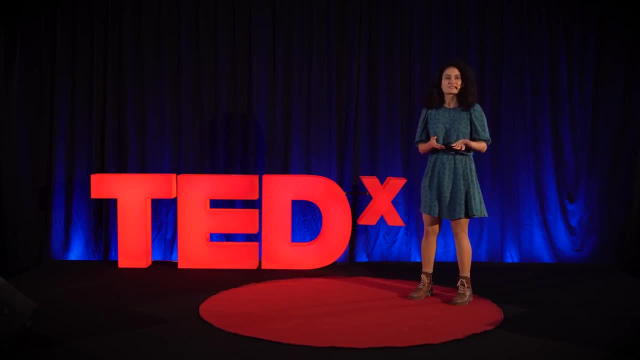 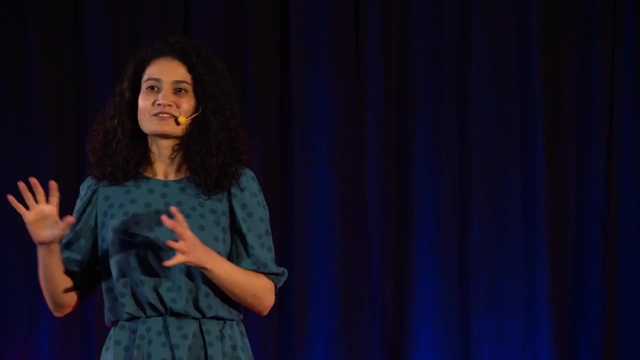 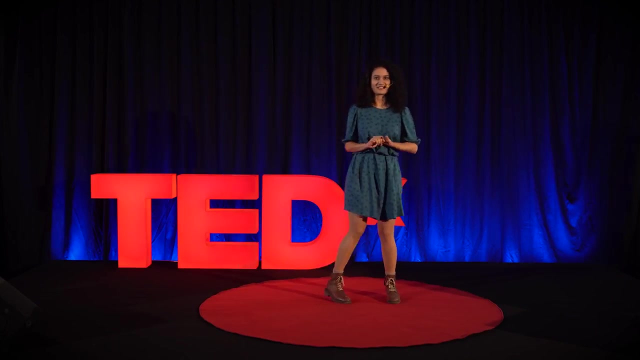 So should we start from research, then That's where we have started. but that is not enough. I imagine you're already drawing this vicious cycle of education science industry axes in your head. If you're getting dizzy, try looking at one spot. I can stand still. 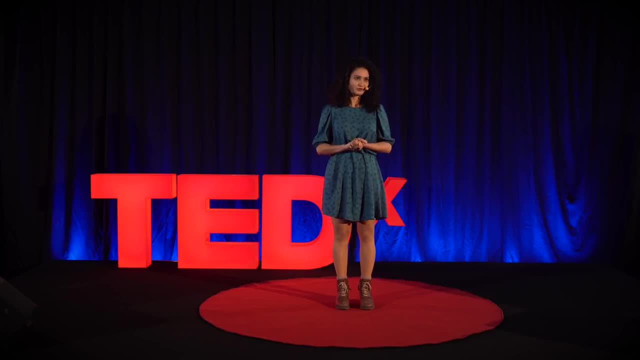 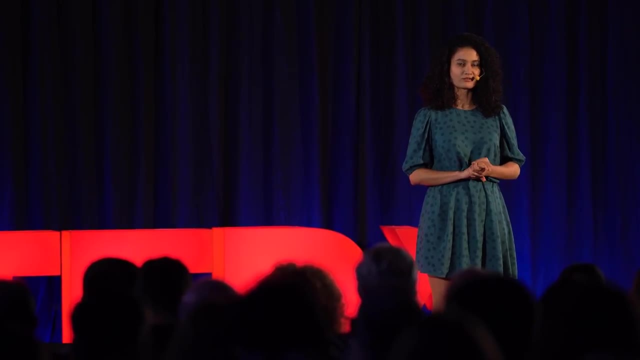 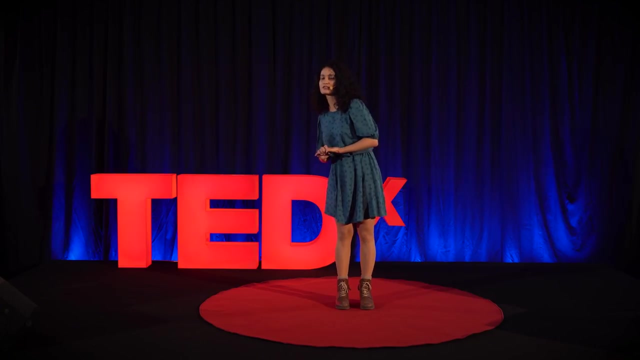 This is a complex problem requiring a complex solution, So you won't hear easy recipes today. Focus on basic science with simultaneous gradual impact on education and industry became our strategy. To implement this strategy, we are creating a culture of communication- Communication between students. 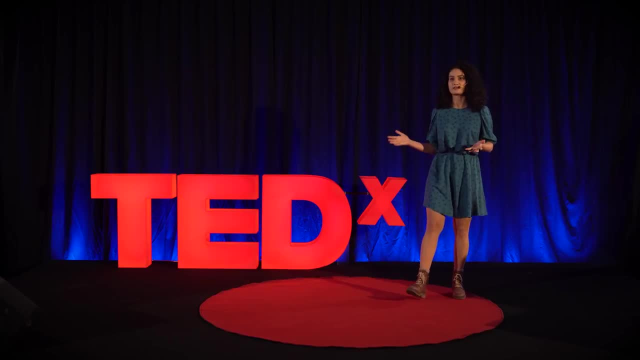 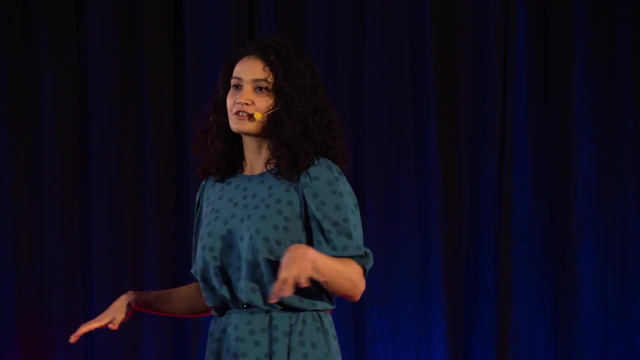 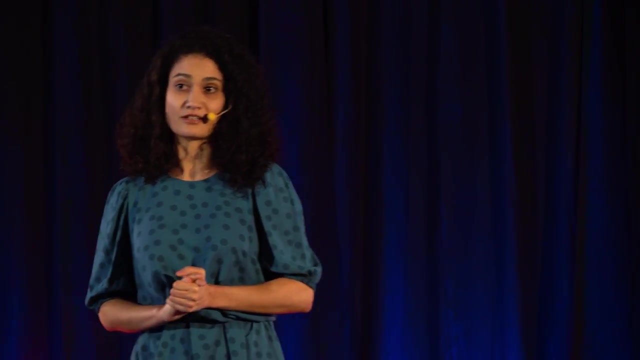 and researchers, between Armenia and abroad, between biologists and data scientists, between academia and industry, between research entities in Armenia. This is because researchers are driven by the scientific environment. Infrastructural and financial resources are needed, but the scientific environment is crucial. 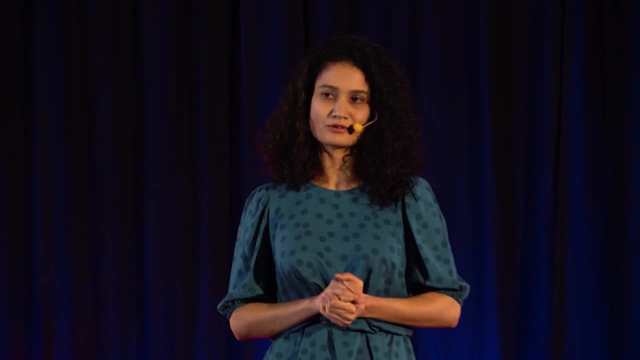 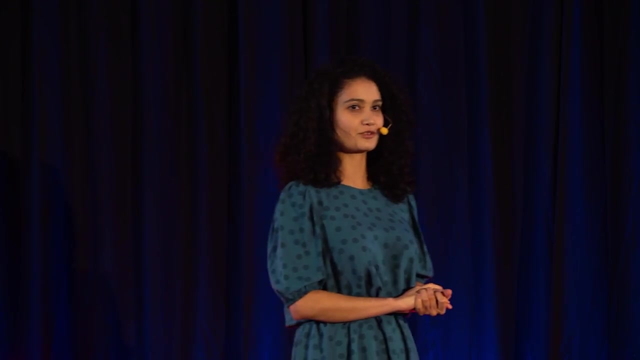 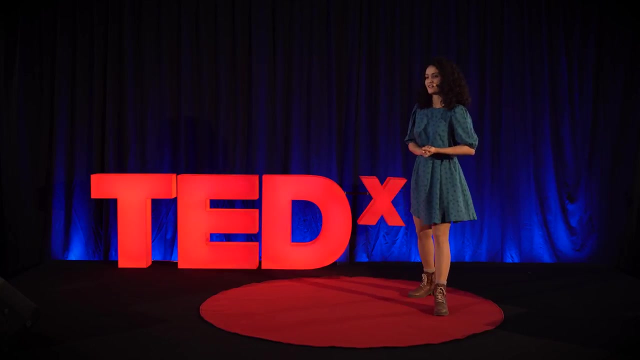 because innovation happens in the corridors, when two different minds meet and talk. And this is what we are trying to achieve with our weekly meetups of various formats, including students, researchers and industry experts from Armenia and from abroad. Next, we are bridging knowledge gaps with non-formal educational activities. 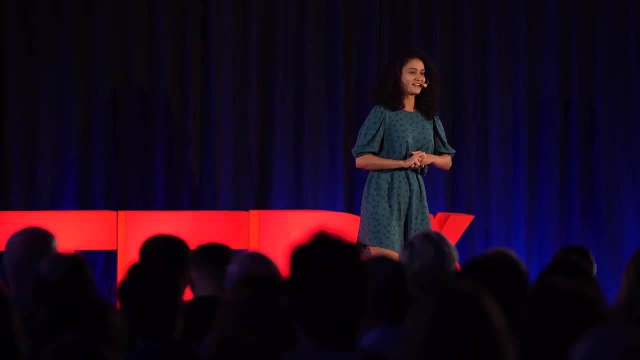 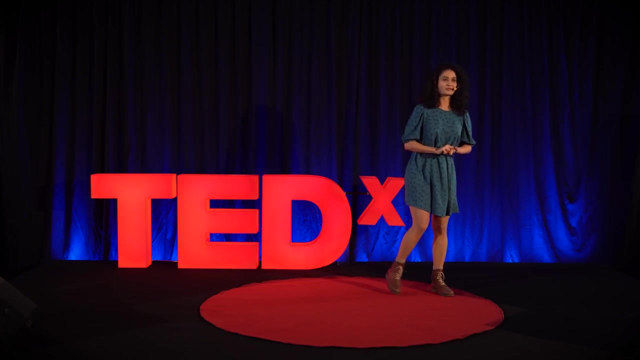 Our big bang summer school this year has attracted the best students to the field by providing a rich content in bioinformatics. due to the hard work of two mentors and participation of 36 speakers from 11 countries, We are proud to tell that we have retention of more than half of these students after the school is over.